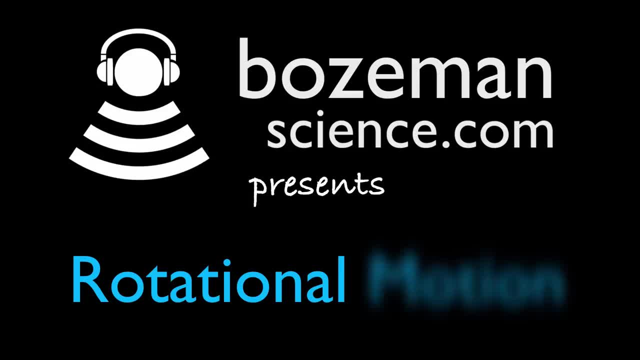 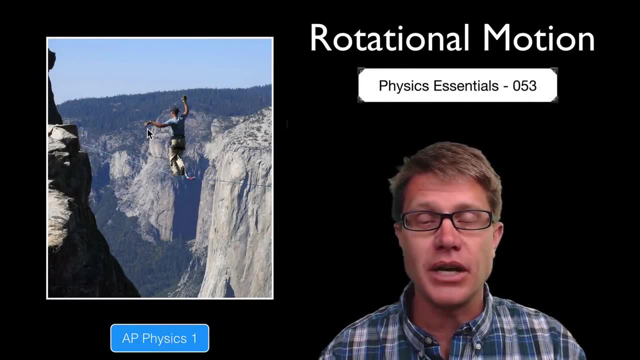 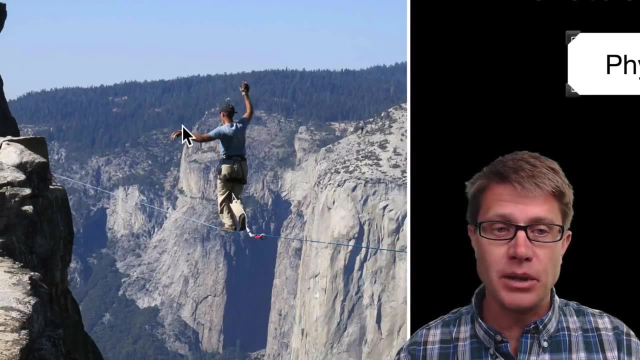 Hi, It is Mr Andersen and this is AP Physics essentials, video 53. It is on rotational motion, which is turning motion, And that would be dangerous. if you are a slackliner, like this person in Yosemite As he applies a force or a net torque on one side, you are going. 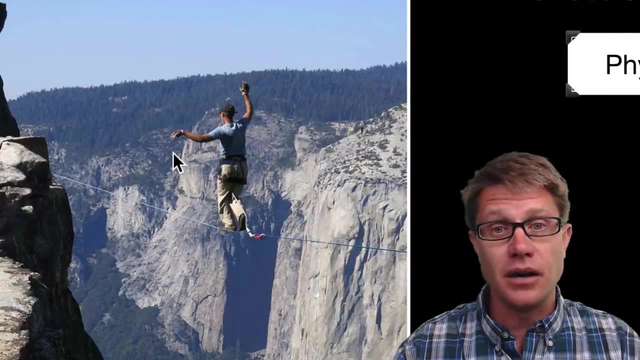 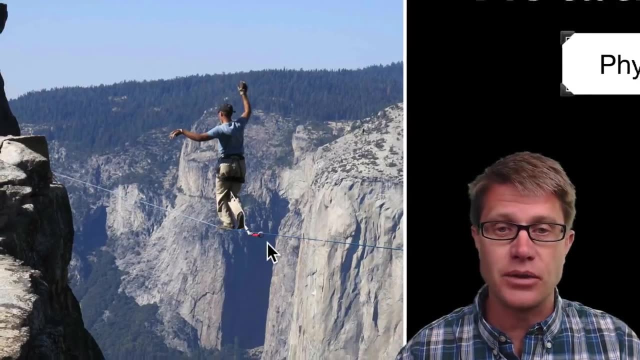 to get rotation, which he has to counteract with a net torque in the other direction, And so by moving your arms out you can increase your inertia, but it still is difficult, And that is why he is attached on here with a rope, And so if we take an object and apply, 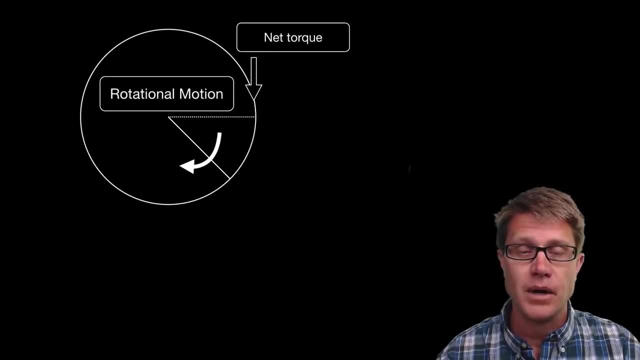 a net torque to it, what we get is rotational motion. We measure that in physics according to its angular displacement, so the angle at which it is turning, its angular velocity, so the speed at which it is turning, and then the angular acceleration, which is how much? 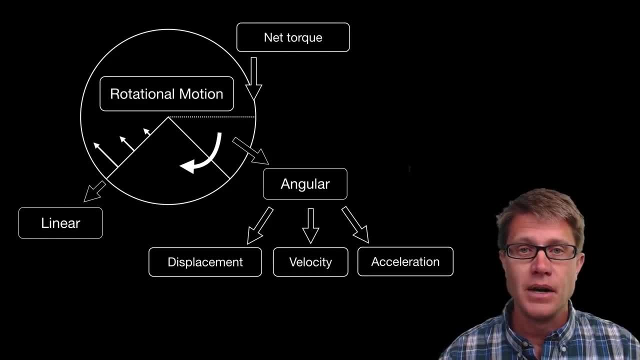 that angular velocity is increasing or decreasing over time. Now the whole object has the same, for example, angular velocity. But if you look at different distances out from the axis of rotation, obviously out here it is going to be going faster than it is in here And 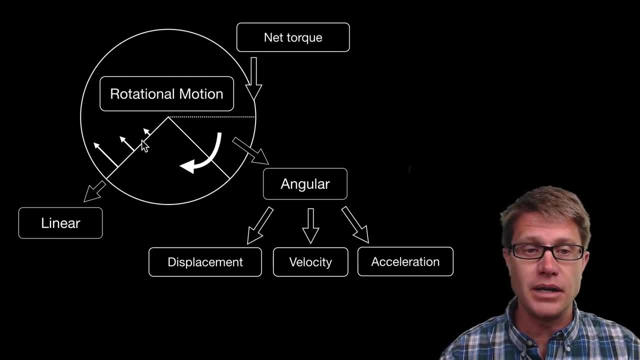 so all we do, for example, is take the angular velocity times the radius or the distance from the center, And that is going to give us its linear velocity, or its speed in that one direction. Now, another term that you should understand is rotational inertia, And so we 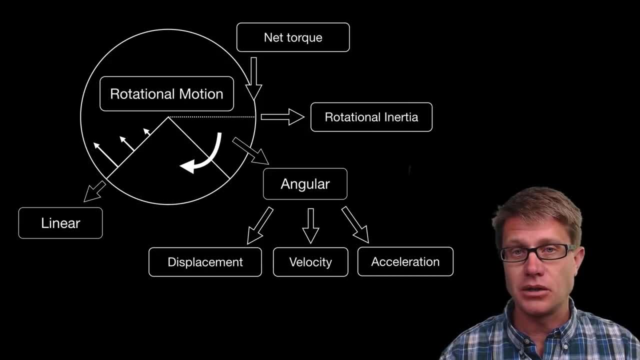 know in regular physics that force is equal to mass times acceleration. If we apply a force times a mass, we are going to get an acceleration. Now in rotational motion, the equation looks a little bit different If we apply a net torque. so if we are applying 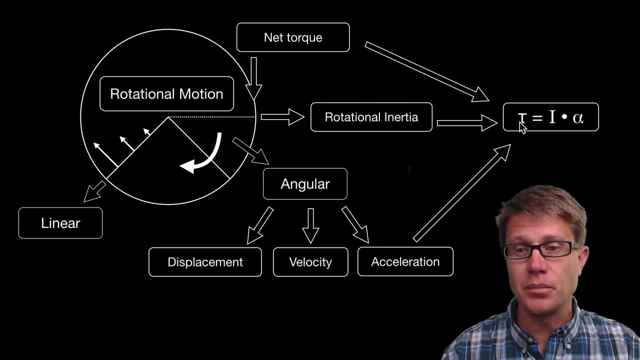 a force, remember, that is perpendicular to the lever arm. if we apply a net torque, that is going to be equal to the rotational inertia. In other words, that is how much this object resists change, or resists that change in motion times, the angular acceleration. And so a good 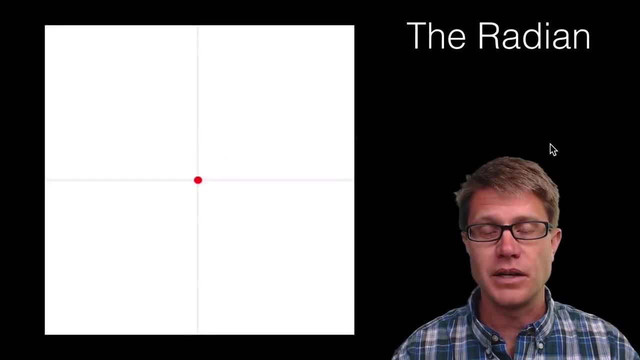 understanding of rotational inertia is important when you are trying to solve problems like this. Before we get to that, we have to understand the importance of the radian, Because that is the base unit When we are measuring angular velocity, for example, or angular acceleration. So, if I 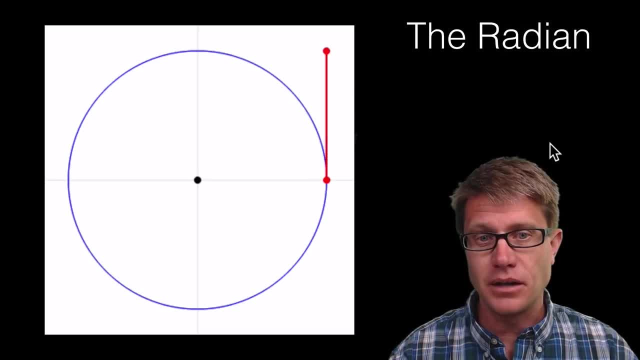 draw a radius like this, and then I take that distance of the radius and wrap it around the circle. I now have the angle of one radian, And so this would be one radian, two radians, three radians. This would be pi radians, 180 degrees, or half a revolution, Or, if we go, 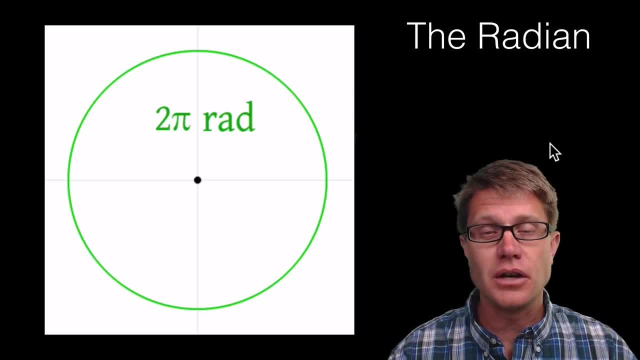 all the way around. that is two pi radians, And so you should understand what a radian is. It is about 57 degrees, But also it is the base unit as we are measuring the angular velocity, this rotational motion, And in the back of your mind you should know that. 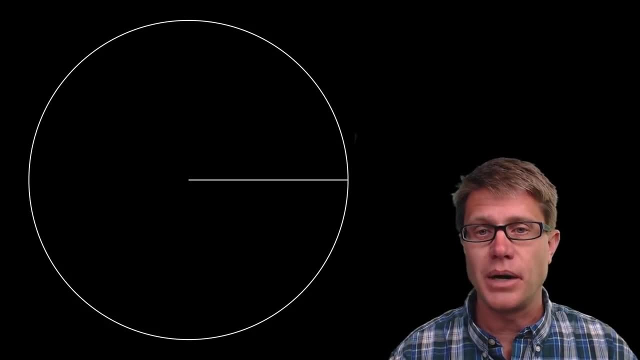 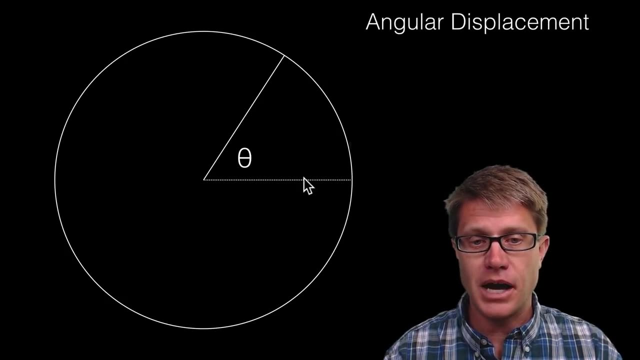 one revolution equals 360 degrees, equals two pi radians, And so for measuring angular displacement, we measure that using the angle theta. So it is going to be how much it is turning, or the distance by which it is turning, And so again, we would measure that in radians. And 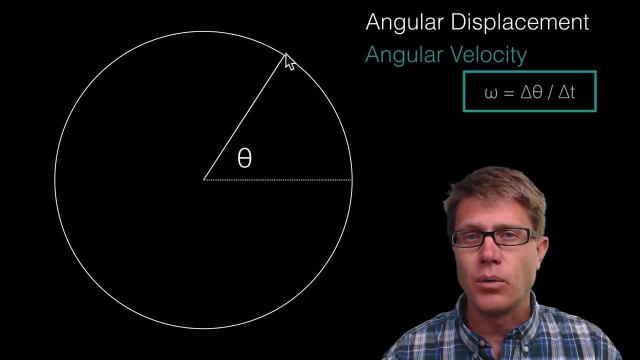 this is one radian. right here It is about 57 degrees. What is angular velocity then? Angular velocity- and we use the symbol omega to represent that- is simply the change in that angle over the change in time. So let me animate this for a second. We are going. 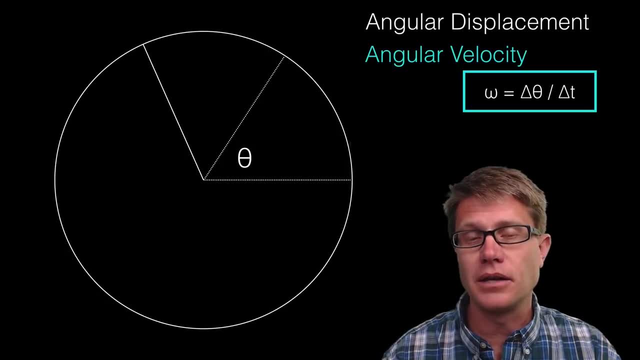 to move that one radian in one second, And so what would our angular velocity be? It would be one radian per second, And so it is how fast this thing is turning. So if it took one second to go all the way around, then it is going two pi r or two pi radians, rather. 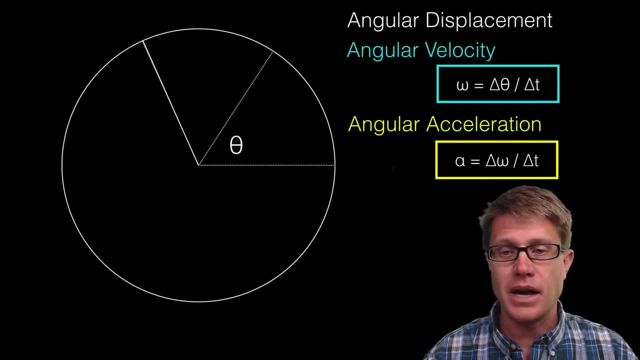 per second. Now let us do an angular acceleration. So what is that? It is the change in angular velocity over time, Or the change in omega over time spinning. At the beginning it has an angular velocity of 0. But after 5 seconds, let's say: 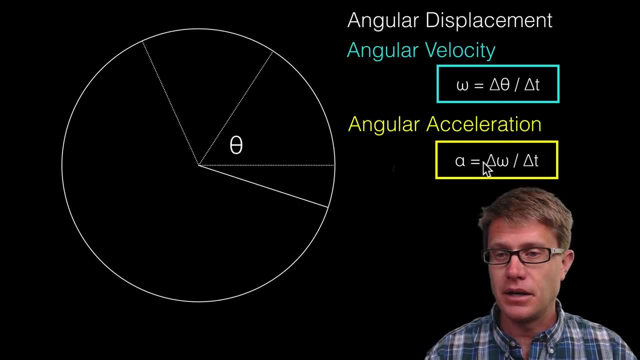 it is going at 1 radian per second. So how would I figure out my angular acceleration? It is going to be the change in omega, which it went from 0 to 1 radian per second. So that is going to be 1 radian per second. How long did it take to do that? It took 5 seconds. 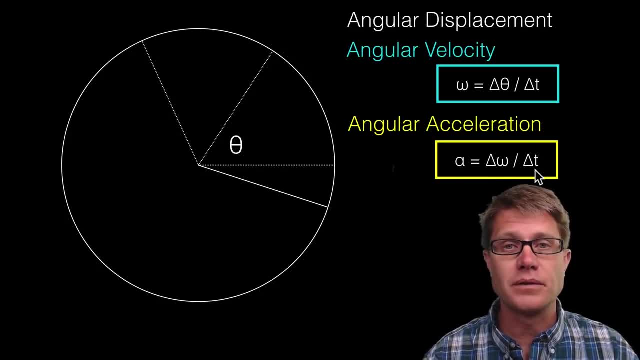 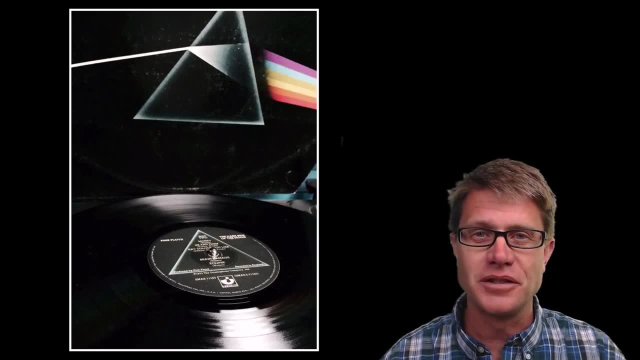 And so my angular acceleration would be 1 fifth or 0.2 radians per second squared. Now let's do some simple problems, And I am using an album of mine. Of course it is Pink Floyd's Dark Side of the Moon. You can see, I have to clean up the album a little bit, But let's. 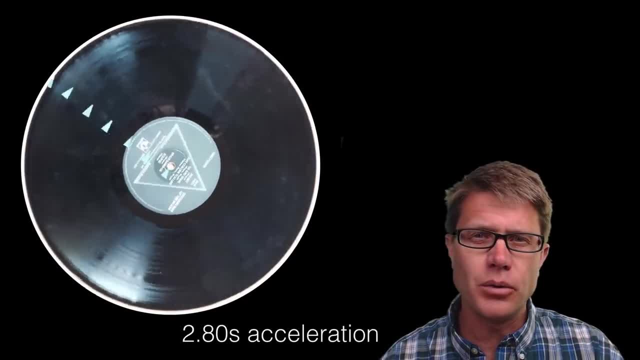 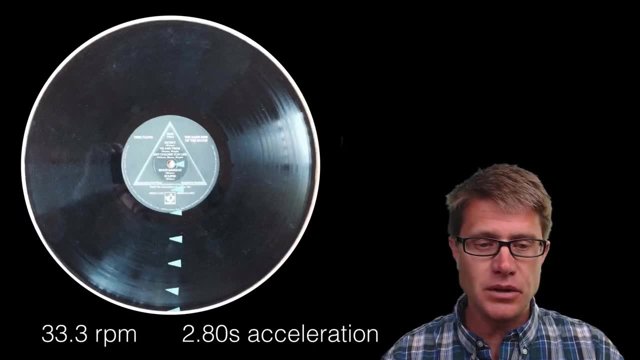 say that I start it spinning like this, And it takes about 2.8 seconds for this to get up to speed, And then it spins at 33.3 revolutions per minute. Well, you can see right away that this revolutions per minute is how much it is rotating in a given period of time, And 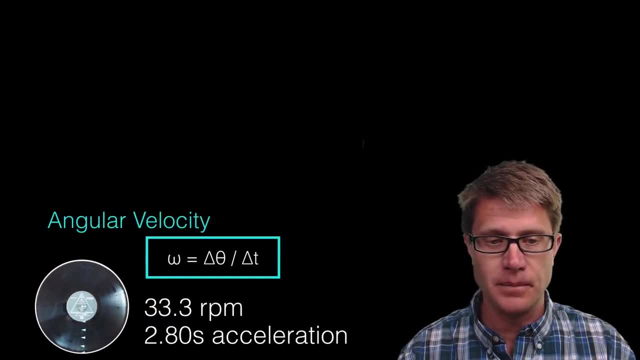 so we are already halfway there when we are trying to figure out the angular velocity. Angular velocity, remember, is equal to the change in theta, So the change in angle over the change in time. And so if I start solving this, what is my change in angle? Well, I said it is 33.3. 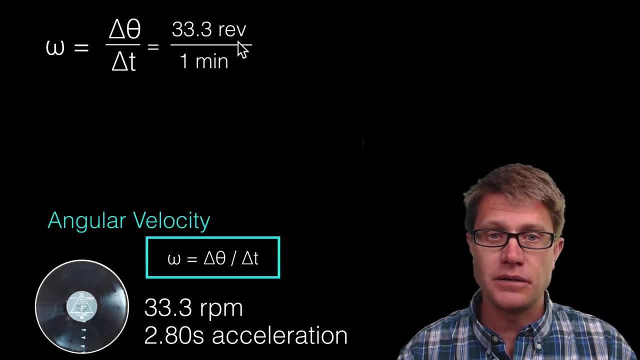 revolutions per 1 minute. Now, these units are bad. We have to get this to radians and we have to get this to seconds, And so we can just do some factor label. I know that 1 revolution equals 2 pi radians, And so right now my revolutions cancel, And I know that. 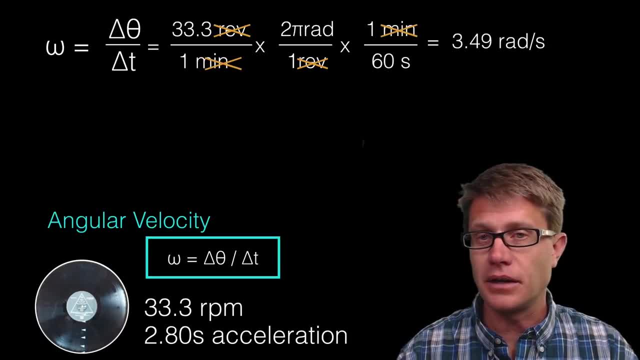 1 minute is equal to 60 seconds, So my minutes cancel And so if I calculate that out, it is going at about 3.49 radians per second, Which makes sense. If it takes a minute to go around 30 times, it makes sense that it. 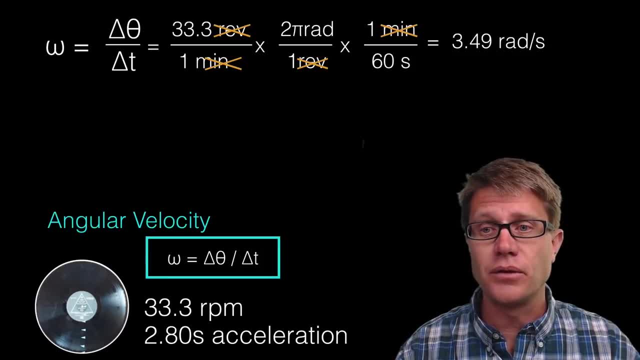 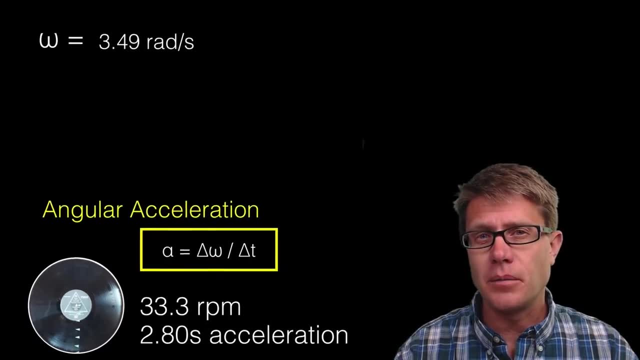 is going a little more than pi radians, or 3.49 radians per second. So that is my angular velocity And it is the same for any point along that album. Let's say I want to figure out my angular acceleration. Now, how do I do that? What do you need to do? Well, I am. 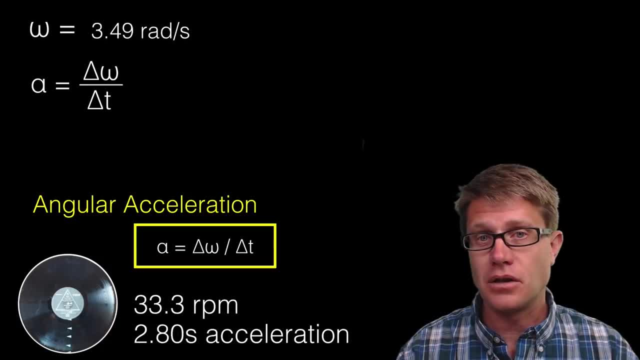 giving you the time at which it is changing, And so it has changed, or my change in omega is going to be 3.49 radians per second, And it took 2.8 seconds to get up to that. It started at 0 and it got up to that speed after 2.80 seconds, And so I am going to get an. 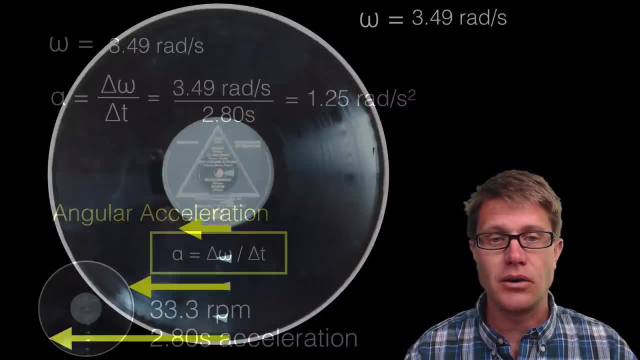 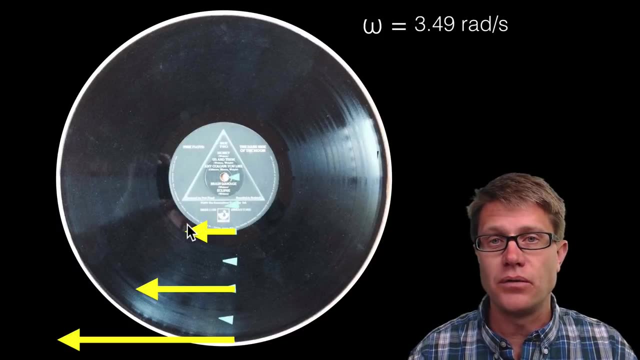 acceleration of 1.25 radians per second squared. So that is how I calculate that. Now, one thing you should understand is that, even though this whole album has an angular velocity of 3.49 seconds, not every point along that album is going at that same linear speed, And so 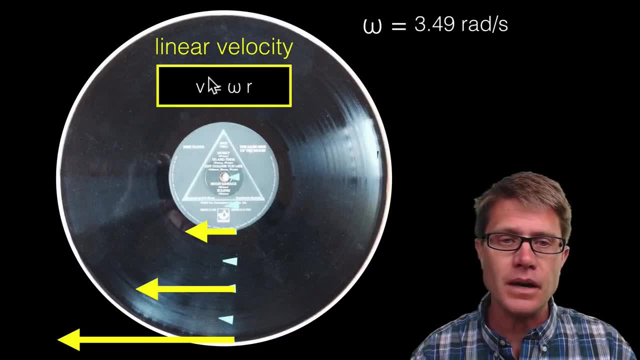 we have an equation for that as well. It is called linear velocity, And linear velocity is 0., And that is simply equal to omega or angular velocity times the radius. And so if we do a point right here in the middle, let's say that is 0 centimeters from the center. 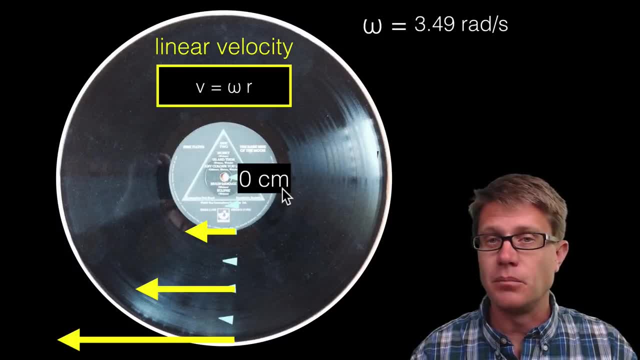 so it is right at the center. Well, there is one problem here. This should be converted to meters, but I do not have to because it is just 0. So if I take my angular velocity of 3.49 radians per second, times 0,, what is my velocity? 0. And so its linear velocity. 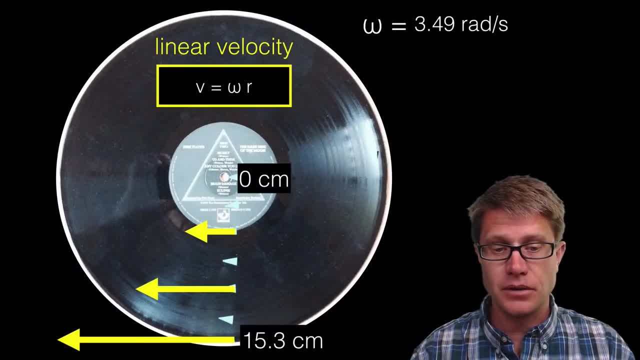 is 0 at the center. What would it be as we move farther out? So let's say out here, since this is a regular album, it is 6 inches out here, or 15.3 centimeters. So if I want to, 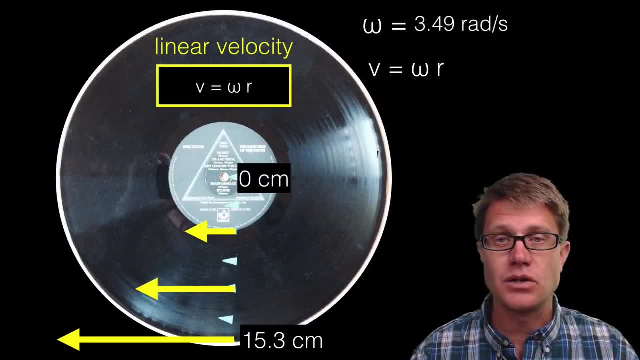 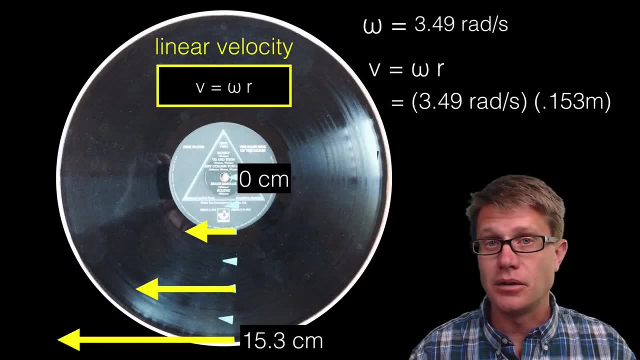 calculate that. I am going to say my velocity equals to omega times radius. What is my omega? 3.49 radians per second. What is my radius? It is 0.153 meters. I have converted that from centimeters to meters. And so what is my linear velocity? 0.534 meters per second. 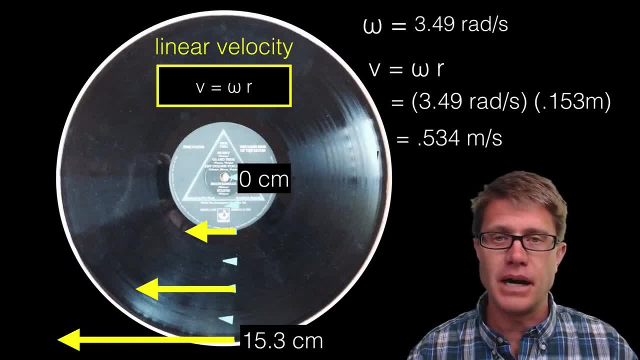 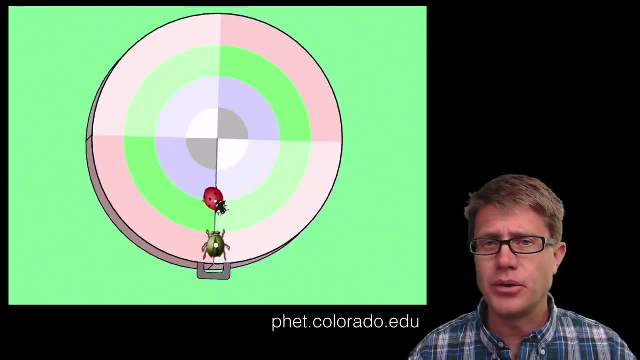 So it is going, you know, a little over a mile an hour if we are going around the outside. So it seems like it is going fast, but not that fast. And now we are going to start talking about applying forces to an object and creating. 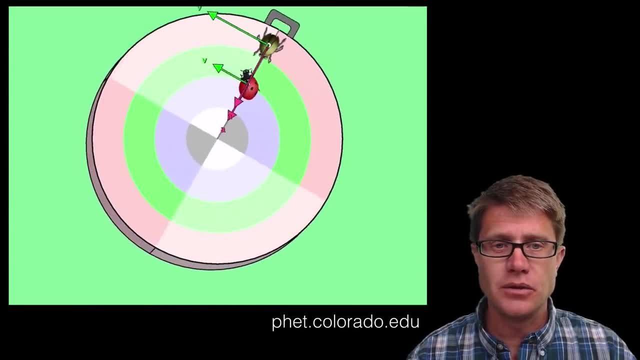 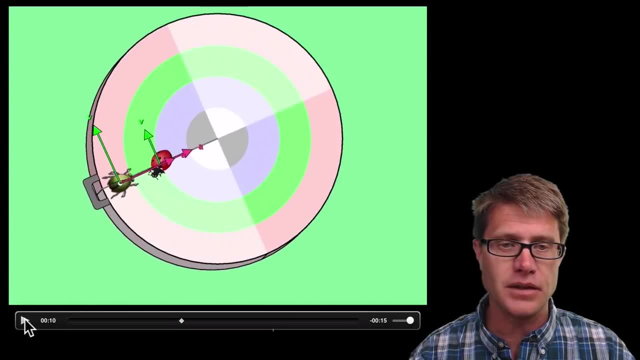 these motions, And so there is a nice PHET simulation. You can see that if I move it in this direction at a constant speed, I have got linear velocity. If I move it in the other direction, I have got linear velocity. Let me freeze that for just a second, And so now. 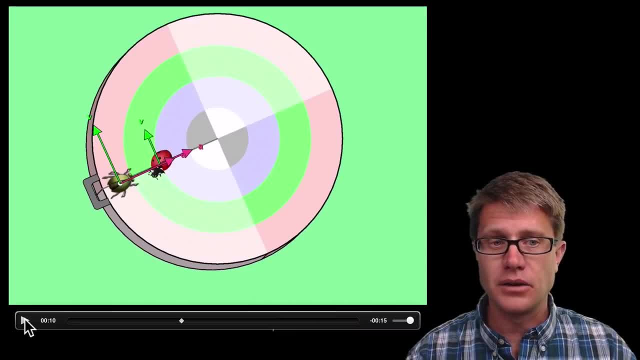 it is not accelerating. It is just moving with a constant angular velocity. But what you can see is the linear velocity is greater on the outside than it is as we move farther in. But also this is accelerating. Even though the velocities are constant, their direction is changing, And so what we have is called a 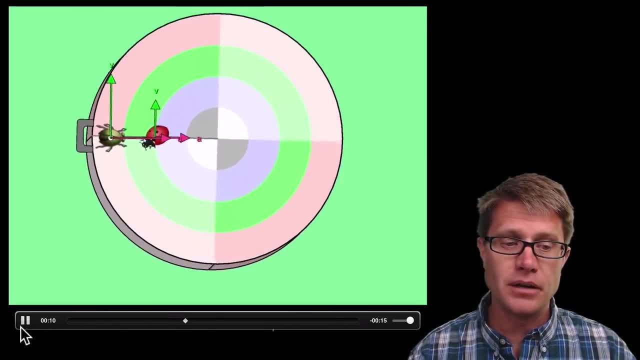 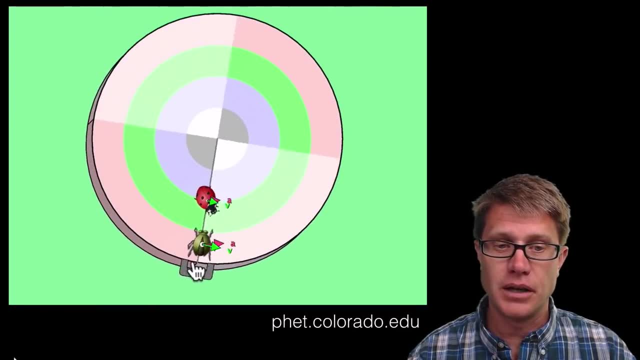 centripetal acceleration to the inside, But what I am now going to do is start applying a net torque to it, And so I am going to start pushing and pulling on it, And what you will see is that we will get huge accelerations in one direction and then, as it stops, it goes. 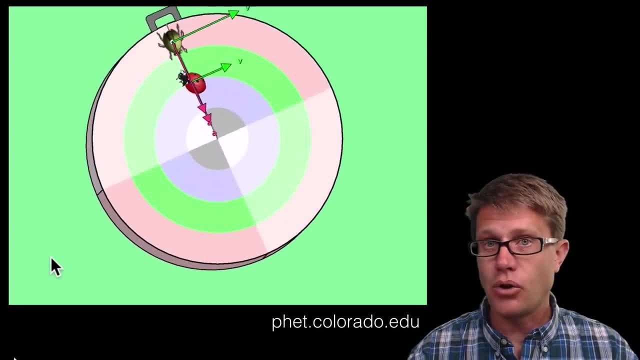 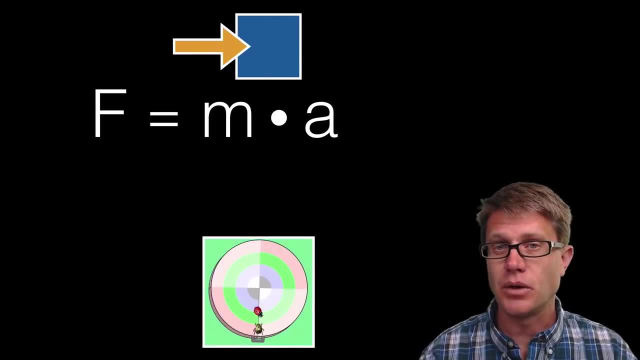 back in the other direction. So as you apply a net torque to an object, we are going to get that acceleration, And so, just like force is equal to mass times acceleration in rotational motion, our torque, or that force that we are applying, is equal to not mass but rotational. 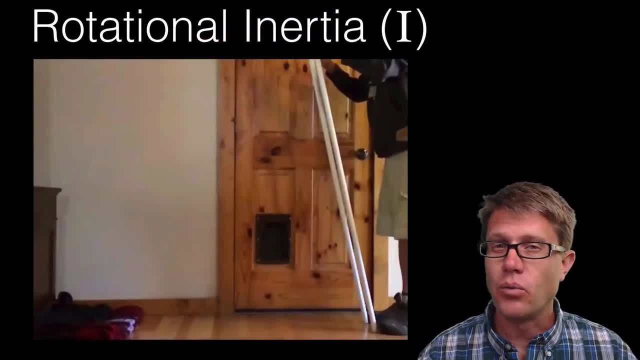 inertia times its angular acceleration. And so what is rotational inertia? Again, it is the resistance to motion of an object in rotation. And so to demonstrate that, I have two pieces of PVC pipe, They are exact same mass, Exact same length, And I am going to drop them at. 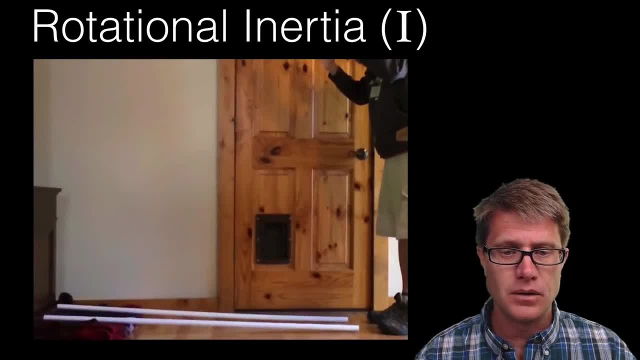 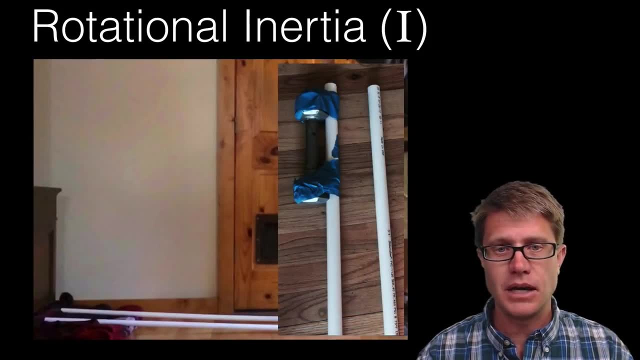 the exact same time, And you can see that they land at the exact same time. Now, what I did is I they taped a weight to one of the PVC pipes and then I am going to drop them at the same time. So make a prediction for a second. Which one do you think is going to land first? The 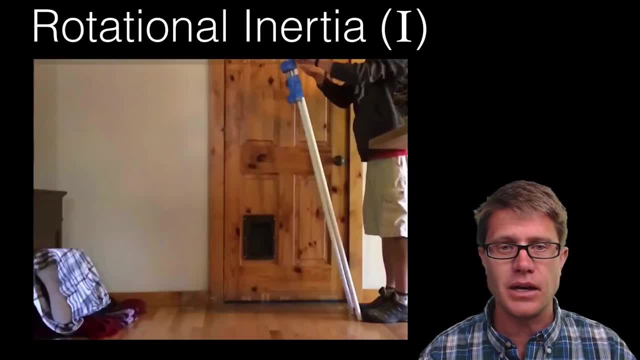 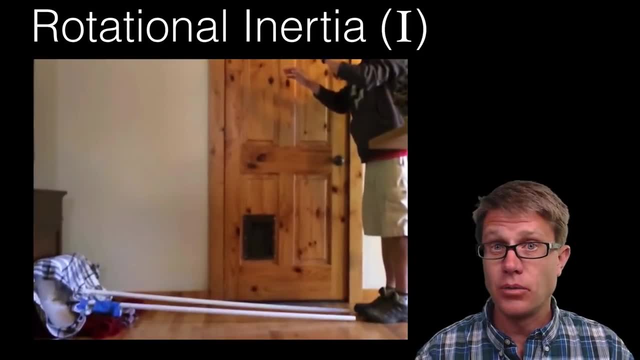 heavier one, The lighter one? Are they both going to land at the same time? Let's let that go, And so you can see that the lighter one hit first. Why is that? It is because it has less rotational inertia And so, as this force, force of gravity, acts on it, it 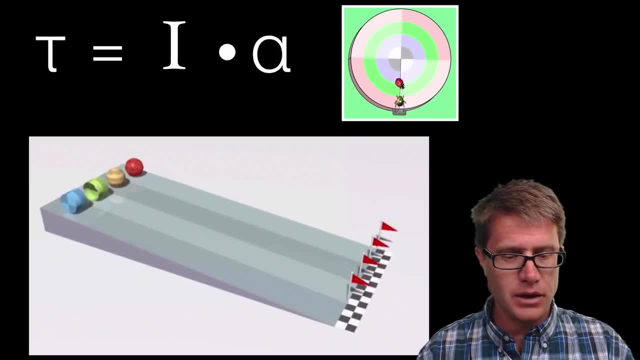 is going to turn with a lower acceleration, And so another way to look at this is a demonstration. here, What I have are four objects that all have the same mass. This one right here is a solid cylinder, And this is a cylinder where all the mass is on the outside. This is a 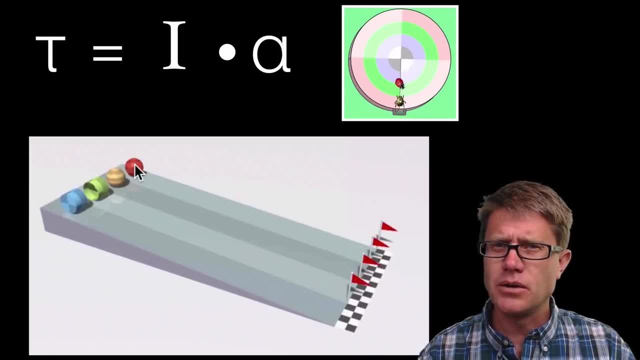 solid sphere And this is a hollow sphere, And so which one do you think is going to make it to the bottom first if we race them, and they all have the same mass, Well, this is kind of counterintuitive as well. If we let this run, you will see that the solid cylinder 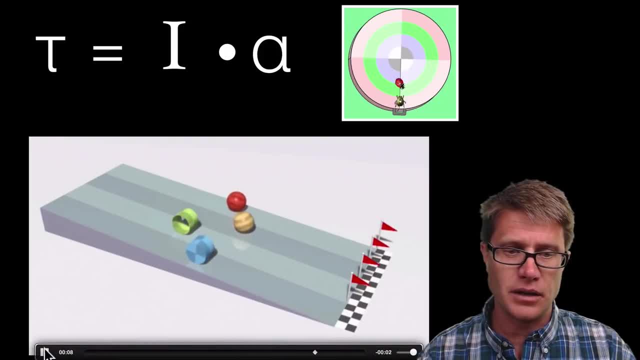 gets there first, And so if we kind of pause that for a second, So this solid, rather sphere is going to make it to the bottom first. Why is that? It is because it is going to have a lower rotational inertia. More of its mass is going to be towards the center of that object, Whereas up here 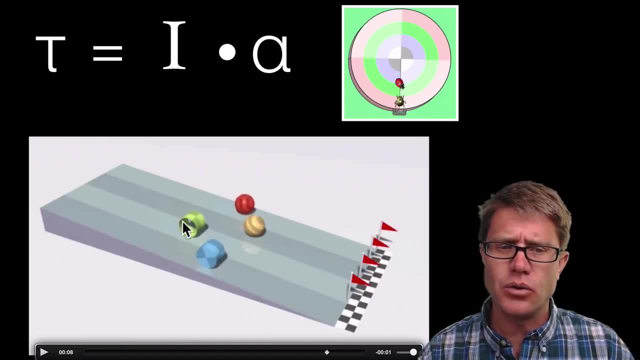 all of that mass is around the outside of the object. Now there are going to be equations to calculate the rotational inertia of each of these, But what you should understand is that the bigger I is, the bigger that rotational inertia is, the more torque we have to apply to have a similar acceleration. And since the force is the 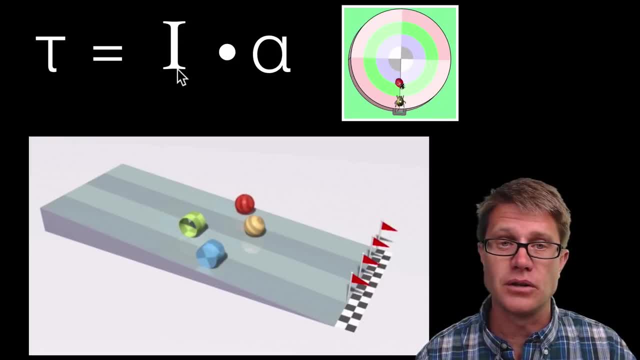 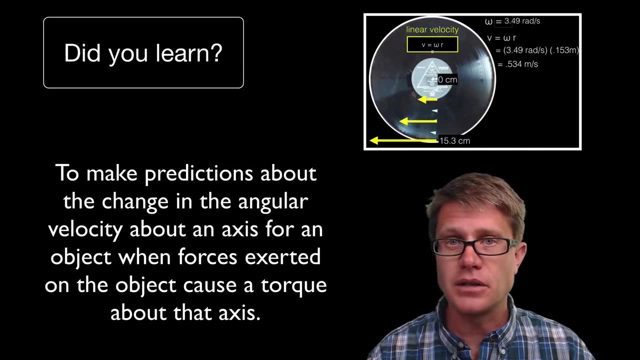 same on all of these: the ones that have the greatest I or rotational inertia are going to have the slowest acceleration. And so did you learn to make predictions about velocity around an object. Again, we have got angular velocity, displacement and acceleration If